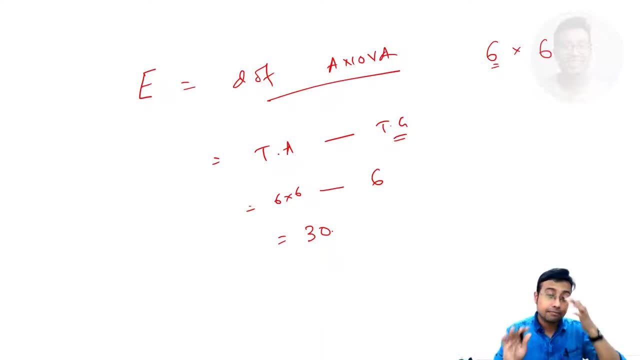 So here it comes to be 30. Right. In another scenario, for example, you take three group, okay, And you take three animals each, So, or you take four animals each, right? So in the total number of animals will be 3 multiplied by 4, equal to 12, okay. 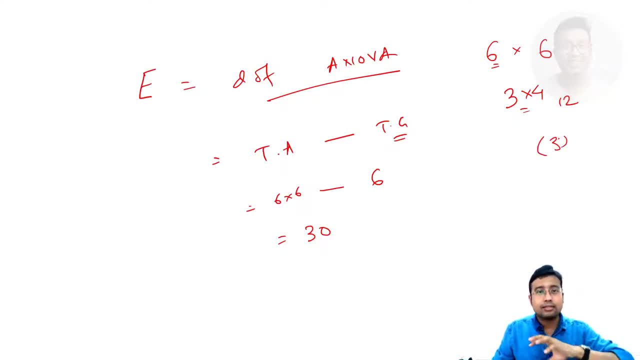 And the group number is 3.. Likewise, I think you already are getting it right Now the important thing that you need to know is: Now, the important thing that you need to know is this: E-value, that is, total number of animals minus the total number of group. 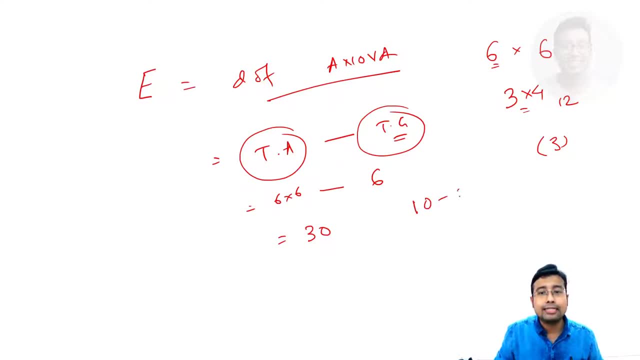 this value should be between 10 and 20.. This is the most important thing. If it is less than 20, then the study is not. statistically valid means whatever you have observed. it may not be applicable to higher population. animal population right. 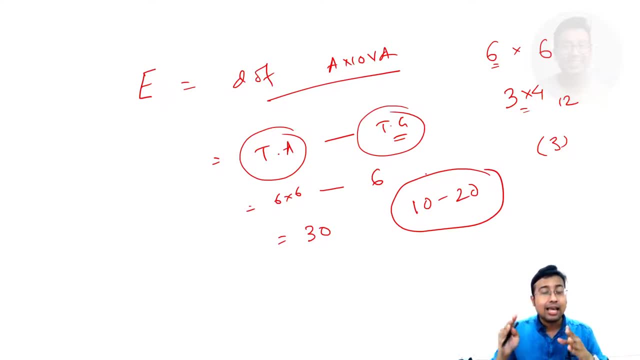 And if it is more than 20,, it means you don't need more than 20,. okay, It should be. if it's more than 20,, then you can. if it's more than 20,, then you can lessen the number of animals. 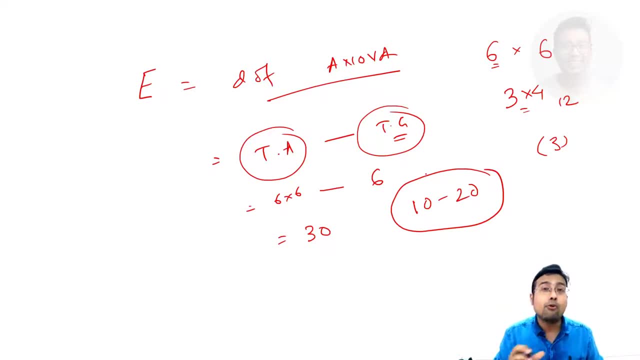 then also you will get the same result. It will not be more statistically valid. So in our case we can see in the first example, 6 multiplied by 6 minus 6 comes to be 30. So here actually we have used more number of animals. 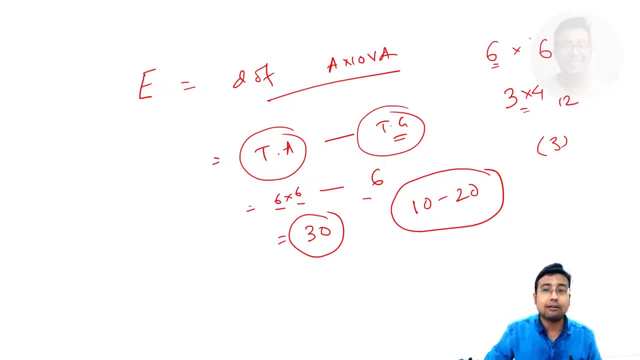 We can decrease the number of animal in each group. okay, Say we can make 5 animals per group, then 5 multiplied by 6 will be 30.. 6 multiplied by 6 is equal to 24, okay, Still it's beyond 10 and 20.. 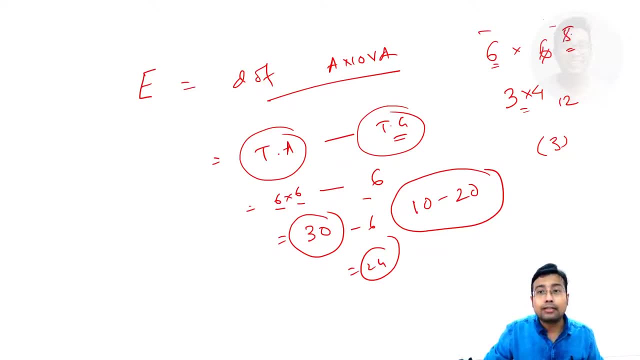 We can still reduce the number of animals, So we need to make the number of animals that is, 4 animals per group. So now it's 24 minus 4, equal to 20,. okay, This is fine. This is the upper limit. 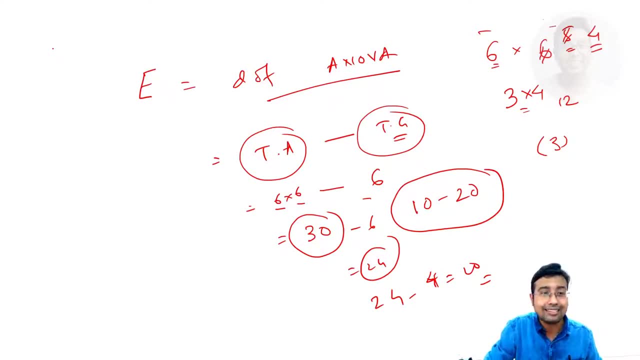 Even you can lessen the number of animals. So let's say now we have 6 groups of 3 animals each. okay, So total number of animals will be 18 and the total number of groups are 6.. So this is 12. This is perfect.